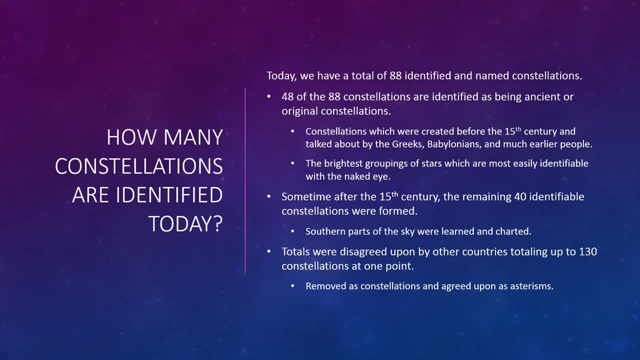 Those stars. So how many constellations do we have today? So there are a total of 88 identified and named constellations. Out of those 88, 48 of them are counted as being ancient or original. Those are the constellations which were created. 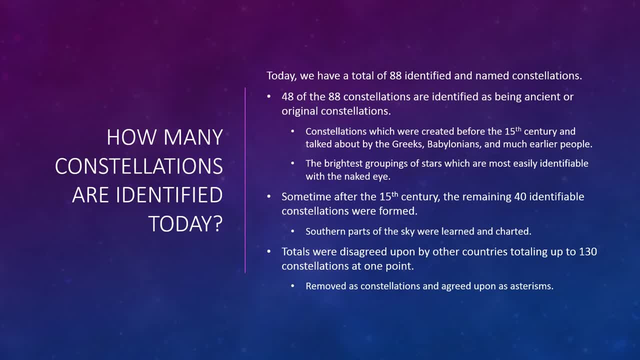 sometime before the 15th century. These were the ones talked about by the Greeks, Babylonians and much earlier people. Anything after the 15th century is counted as a newer constellation, so the remaining 40 are newer constellations which were created after the 15th century, and this 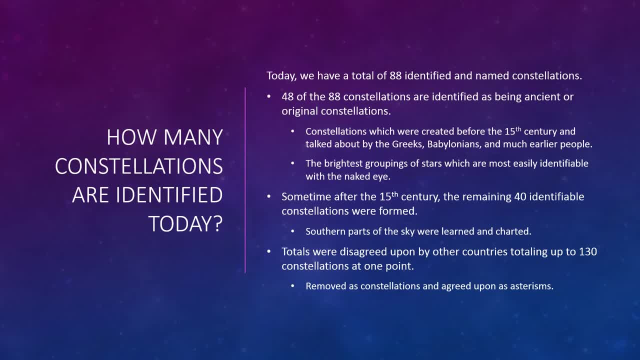 was because before the 15th century southern parts of the sky were not even known about. so after the 15th century we were able to get the technology to be able to learn about the southern sky and what was going on there. the original 48. 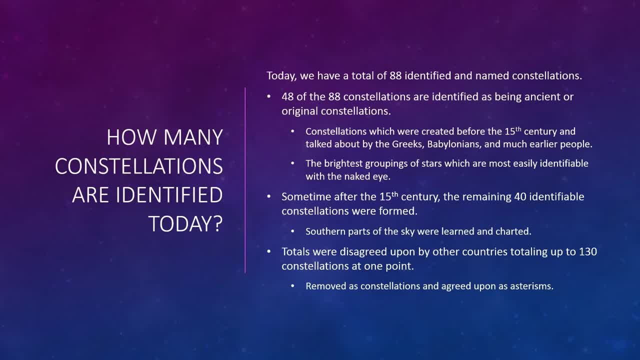 constellations are the brightest ones, so they're the most easily identifiable ones. originally, the totals of constellations were disagreed upon by each country's. at one point there were a total of 130 constellations, but then they agreed to remove those and call them asterisms instead of. 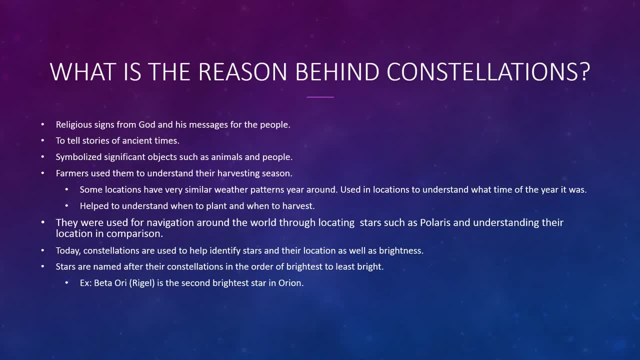 constellations. so what is the reason behind constellations? so there, many people in the ancient times believed that they were messages from God for their, for his people. they were also used to tell stories of ancient times, symbolized significant people and animals, and then farmers used them to understand their harvesting seasons. so 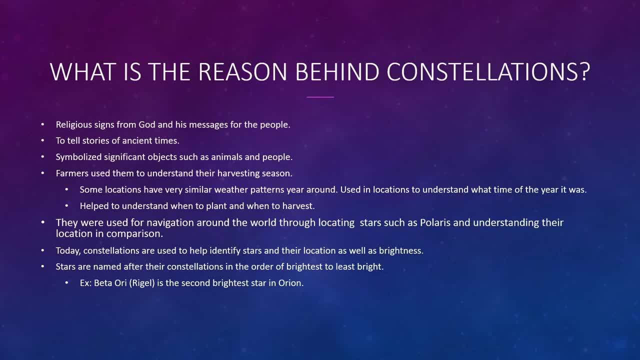 this was because some locations had similar weather patterns, so they weren't sure when it would be technically winter or fall or spring, so they used the constellations to understand what time of the year it was, in order to understand what time of year the year is. 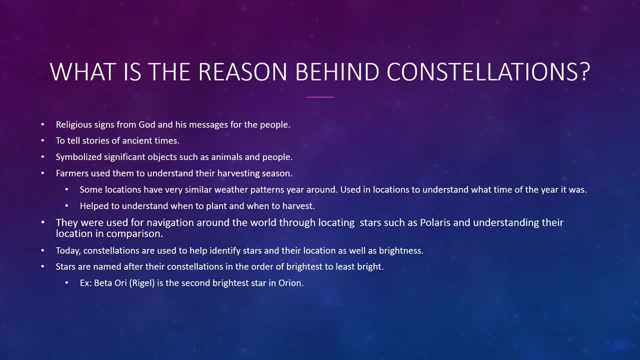 understand when planting and harvesting would be, since certain constellations are only visible at certain times of the year, which we will get into. They were also used for navigation around the world. Another example: with Polaris, understanding where it is, you can use that in location to in comparison to. 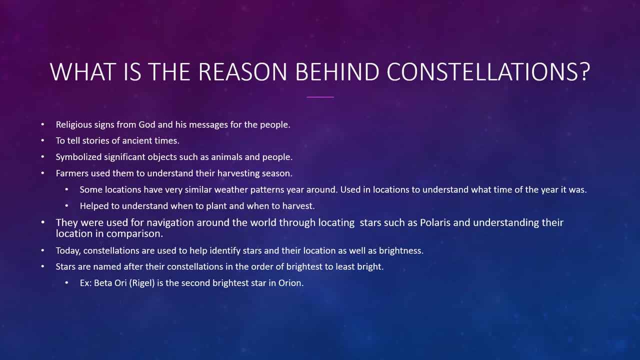 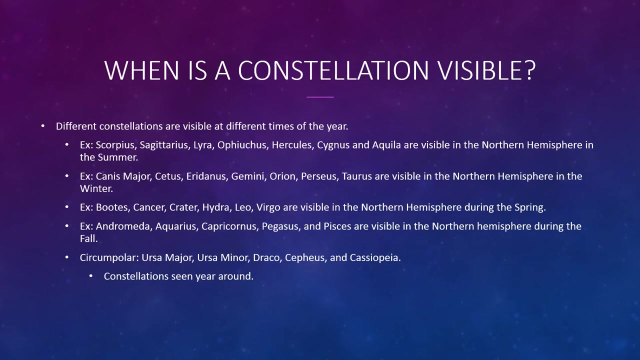 your location. Also, today, constellations are used to help identify stars in their locations, as well as brightness, so all stars are named after their constellation. so, for example, Betoauri is the second brightest star in Orion. So when is a constellation visible? 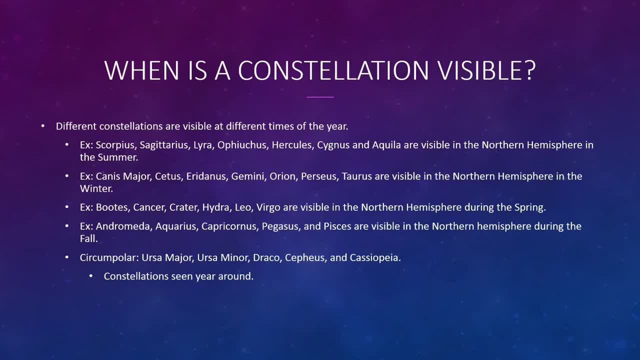 Different constellations are obviously visible, but they are always one second brighter than others. We can see with the at different times of the year, and these are just kind of some of the examples of when they're all visible. and all of these ones are some of the original 48. 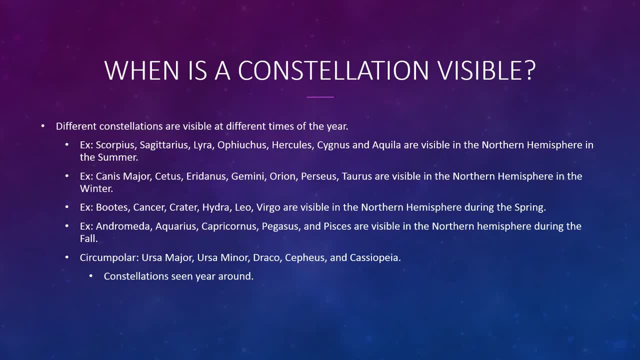 so some of them are obviously visible in summer, winter, fall, spring. any that are circumpolar, such as Ursa Major, Ursa Minor, Draco, Cepheus and Cassiopeia- those constellations can be seen year-round. this is just an example of a summer sky. 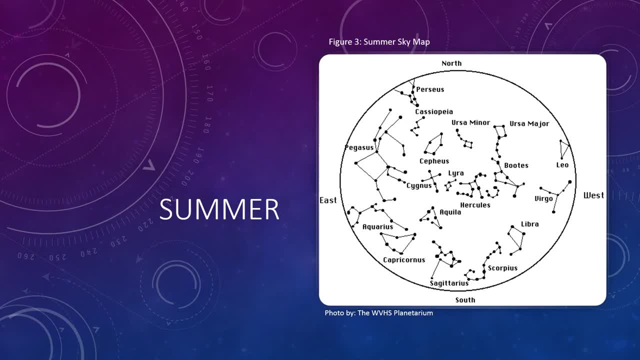 map, kind of to put those that last slide into perspective, of when you can see some of these constellations and kind of where they're at. so, as you can see, some of the circumpolar ones are on there and will be on all of them, but then you've 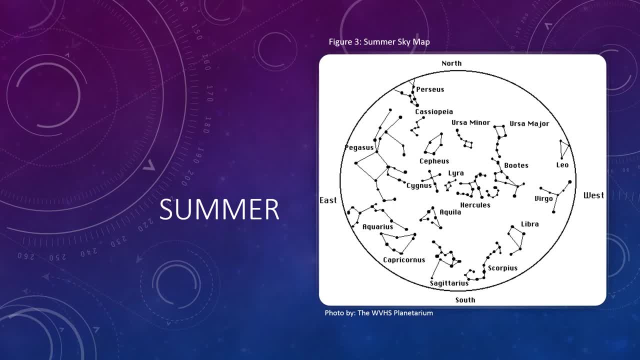 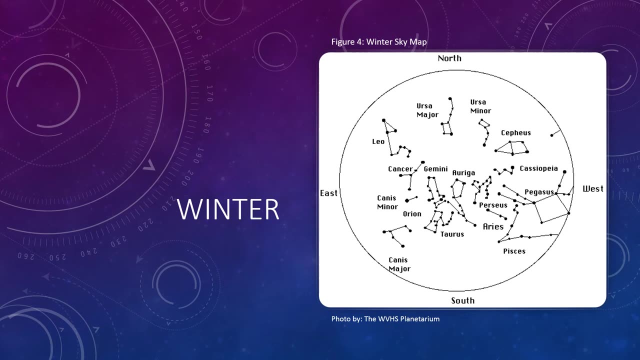 got like Hercules and some of those other ones that are more so only seen in the summer and as transitioning into fall. this is the winter one again, just to kind of show you the ones that are visible during the winter time. all of these ones are also the original 48, so any of these ones shown on these sky maps are the original 48. 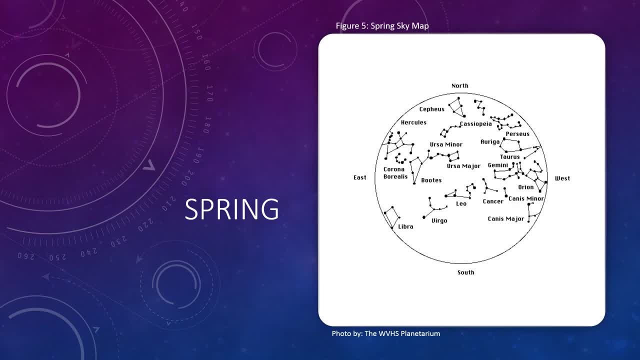 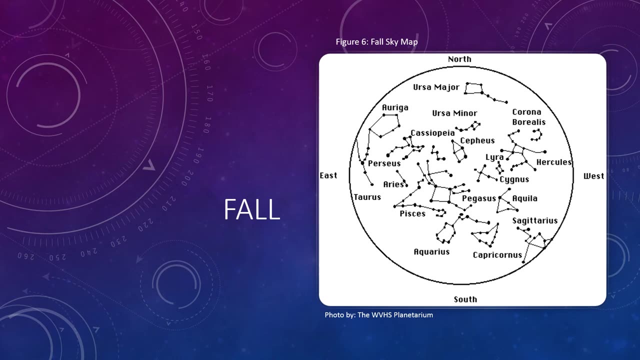 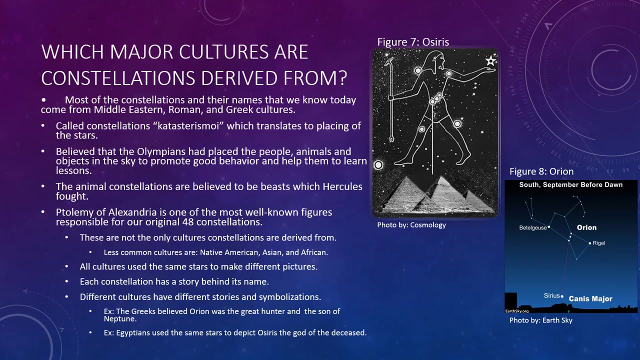 this is spring again. you see the circumpolar ones, but you also see the ones that I listed that are visible during the springtime. and finally, this one is the fall one again, just kind of a visual to put that last slide into perspective. now to move on about which cultures. 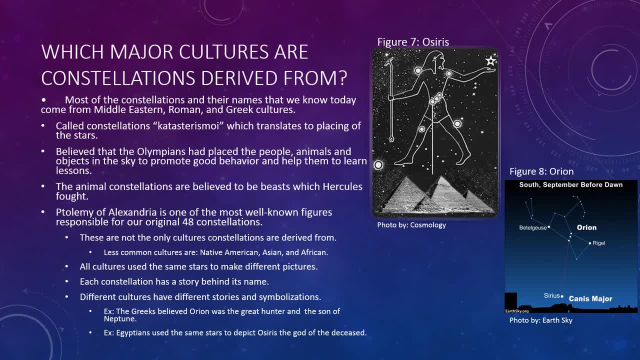 these constellations were derived from. the three main ones are Middle Eastern, Roman and Greek cultures. it's believed that the word constellation was translated to the placing of the stars. that's what the Greeks believed, and they also believed that the Olympians had placed the people, animals and objects in the sky in order to help people to learn. 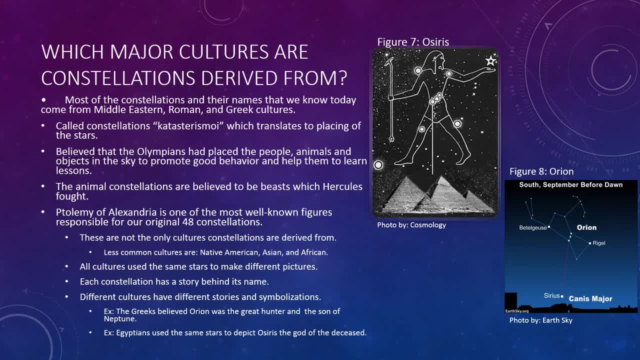 their lessons and to promote good behavior based off of these stories that each constellation would tell. any of the animal constellations are believed to be beasts in which Hercules fought. obviously, these are not the only cultures that constellations are derived from, but they are the main ones. the less common cultures are Native American. 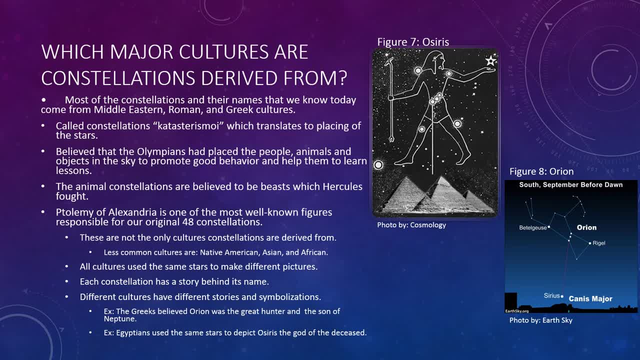 Asian and African, but all cultures are almost above the British one. even sean george is not included, with the Hercules River used the same stars to make different pictures, so not every culture had the same constellation or story behind it, but each constellation has a story behind its name. 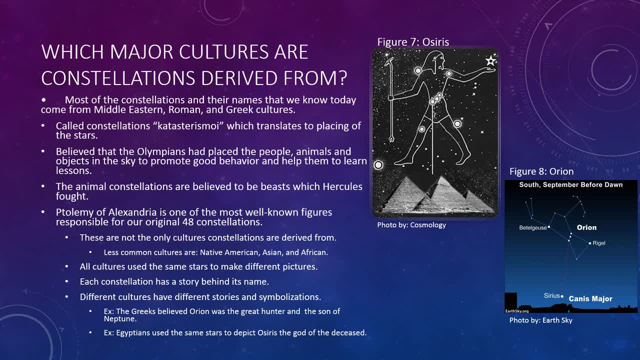 So, as you can see in the picture, we first have Osiris, and that is a constellation named by the Egyptians. Osiris was believed to be the god of the deceased. We are more commonly known to see Orion, and that's the Greek one, and he's the great.